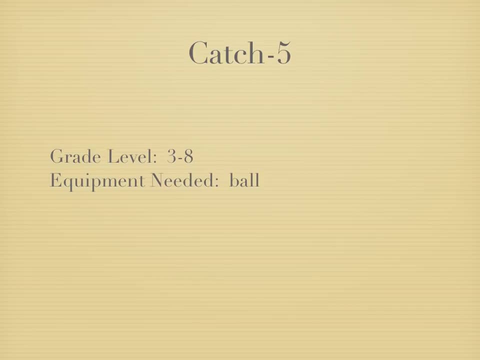 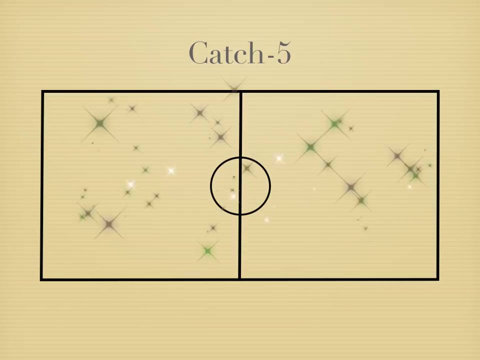 This is Catch Five. It's a game that works on passing and receiving. A friend of mine showed me it this year and we used it in our handball and basketball units and it worked really well. So all you need is a ball. So in this game, you have one team there, the other team against them and they're all spread out along the floor. 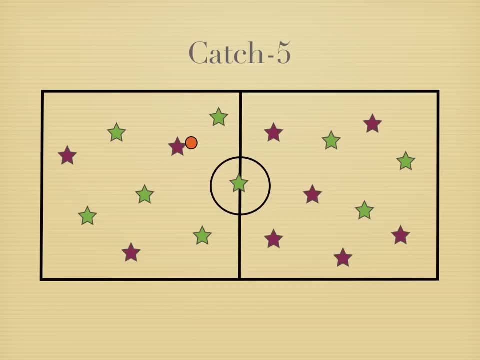 One team will start with a ball. They can rock paper scissors or whatever you want to decide who starts. Essentially, the idea of the game is to try to complete five passes without dropping the ball or without having the other team intercept the passes. 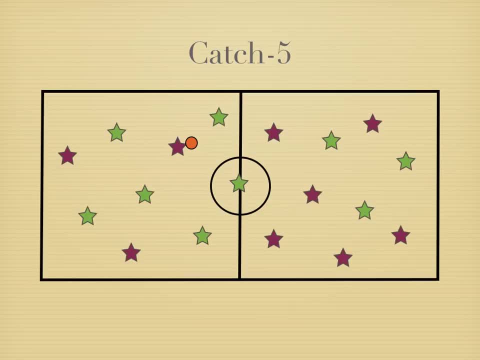 So it's a game that gets players to move to open spots and find the open areas and work on their passing accuracy. So in this first example we'll see one team passing the ball around and it's easy when no one's moving, But obviously in the real game everyone's moving around. 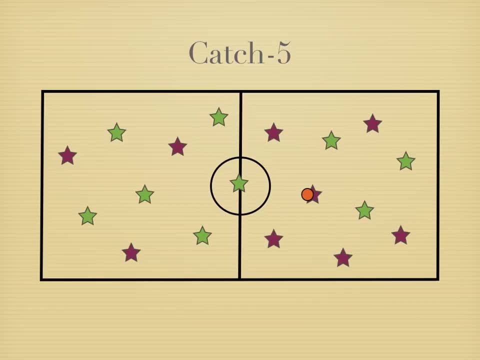 So they've completed five passes there, and on the fifth pass they can put the ball on the ground or slam it on the ground and they get a point. Then the other team would start out with it. So there was just a very quick example. 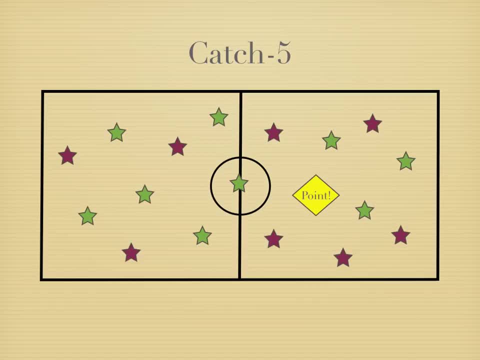 Players can't pass back and forth between two people. You have to pass to somebody else, So that way more people get a chance. So in the second example here we'll see a player goes to make a pass and it's intercepted, So obviously on a straight interception. then the other team gets the ball and they can continue passing it along and try and make five passes. 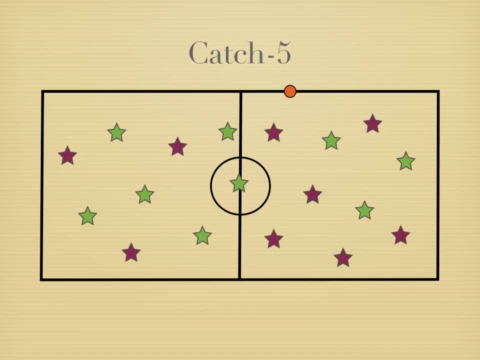 Again, everyone would be moving around. There, we see, a player threw it out of bounds. So when that happens, then it's easy. It's simply the other team's ball And then it continues on, So they can work on pivoting and moving around and all those types of things. 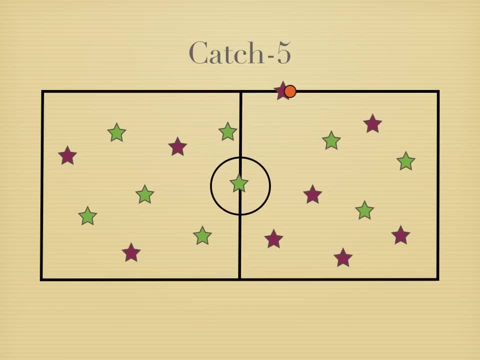 If a team can kind of intercept it, but instead of catching the ball they just knock it to the ground, then the team that knocked it to the ground will also gain possession of the ball. So there, you can implement rules as you see. Thanks for watching. 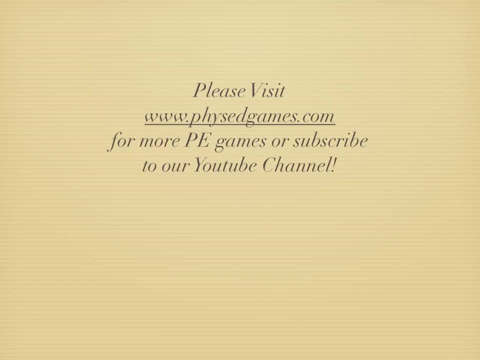 Please visit physedgamescom for more games or subscribe to our channel.